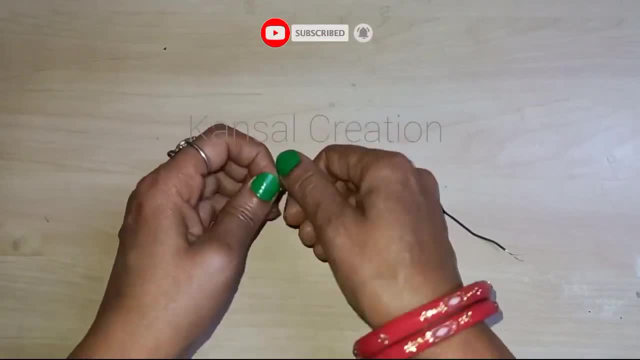 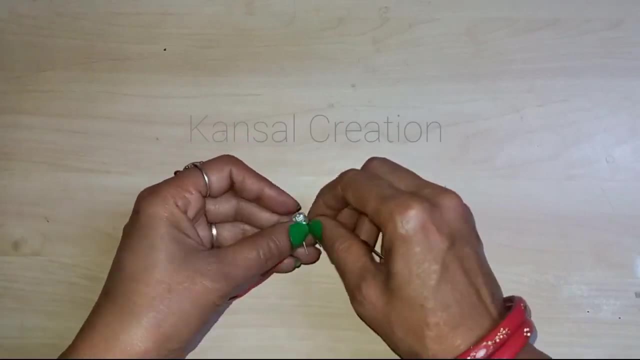 Hustle, hard, hustle every single day. I'll be making moves till I'm buried in my grave To the system. I don't wanna be a slave. I've been doing shit my way for the highway And in the driveway. it's a nice range, Cause I grind through the climb. I invite pain. 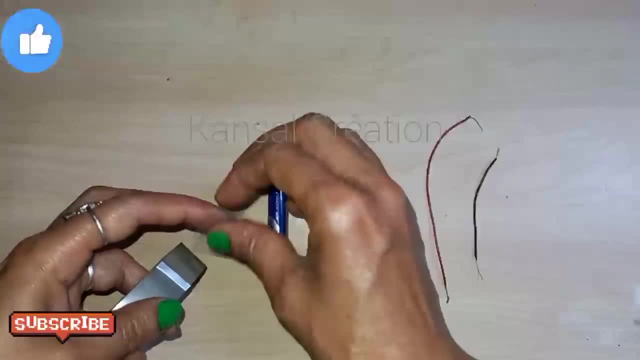 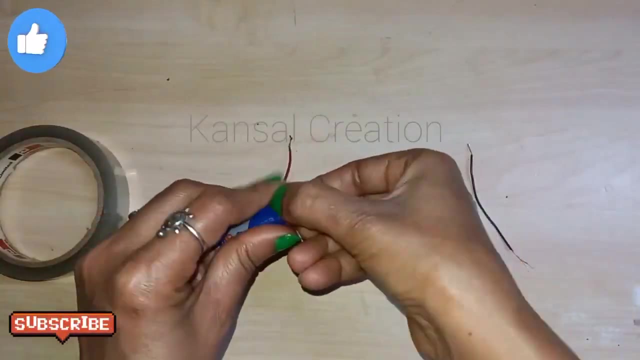 You'll never hear me bitch. nah, don't complain. Just gotta flip the switch and you can go and obtain Anything you want, anything you need. Your mind's got the key ingredient. it's belief. Better see with the negativity, But I just slide right by that energy. 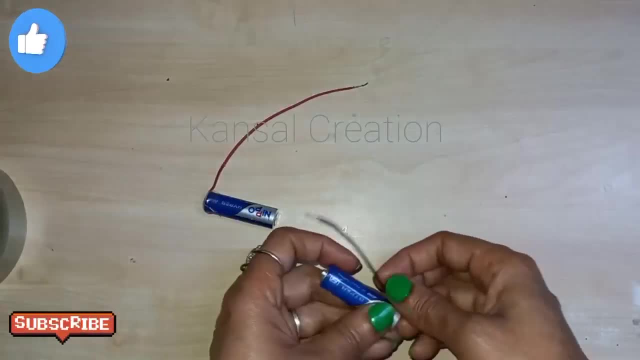 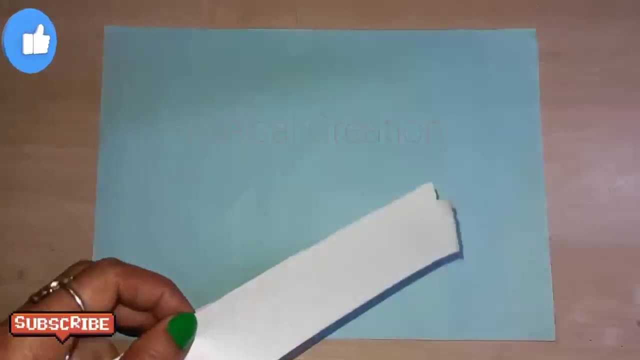 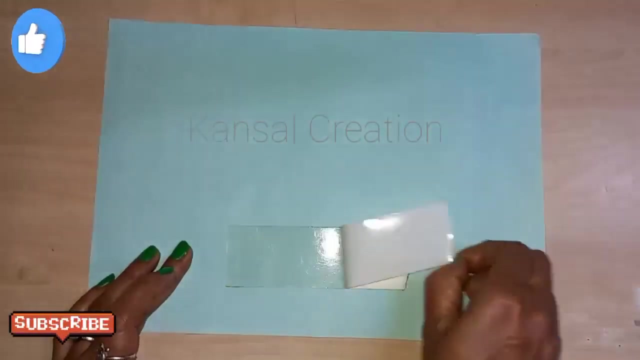 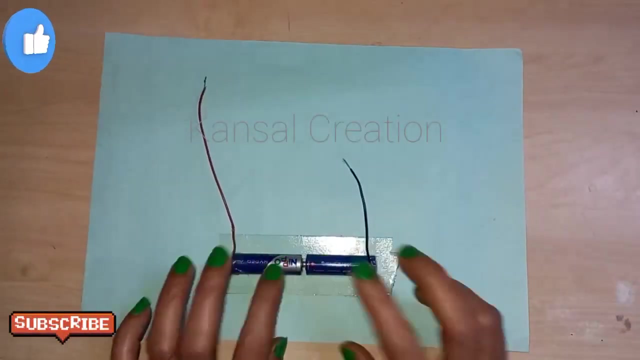 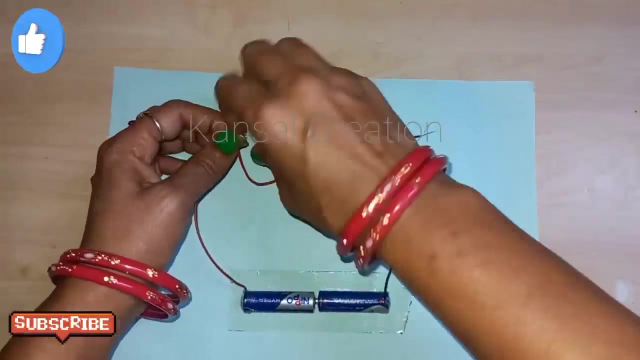 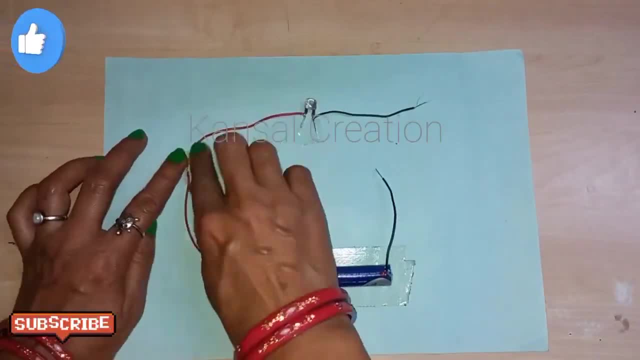 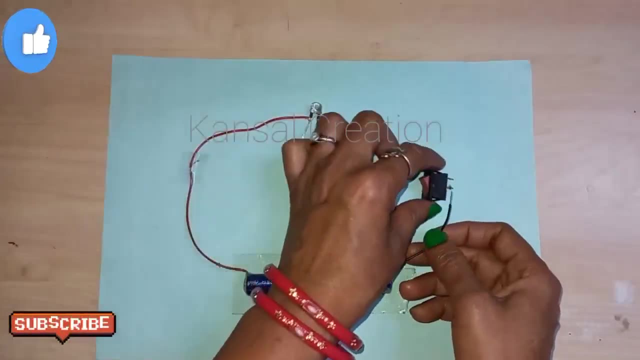 You gotta mind. But even that could change. you could flip the gray matter like some batter in your brain. That's what I say: fake it till you make it A, And if you play that game then you just might make a change. Rearrange all the bad to okay. 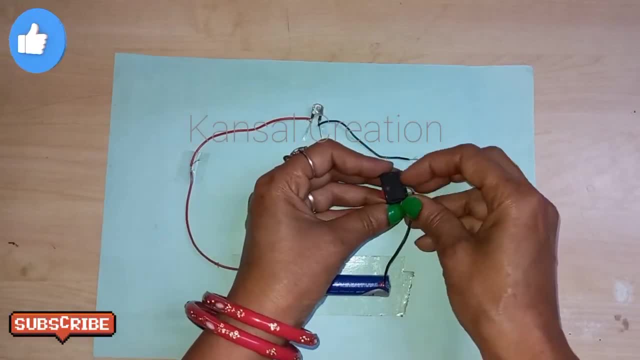 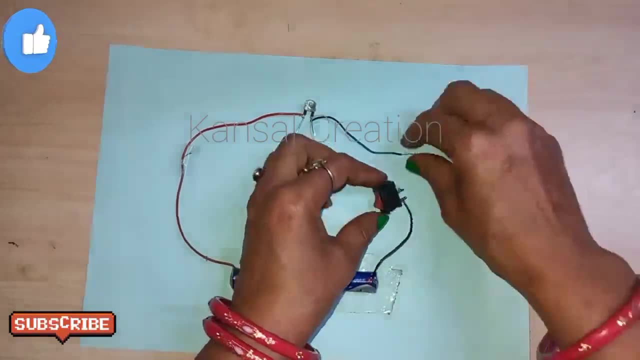 Take the worst thoughts, say them, turn them to a game. Take the best thoughts, say them, put them on display. Don't repeat in your brain till you're feeling no more pain. Never slow yourself down. you can do some more. Push past all the pain and you'll find the door. 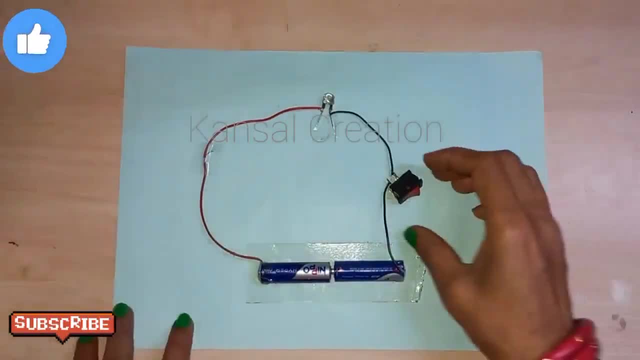 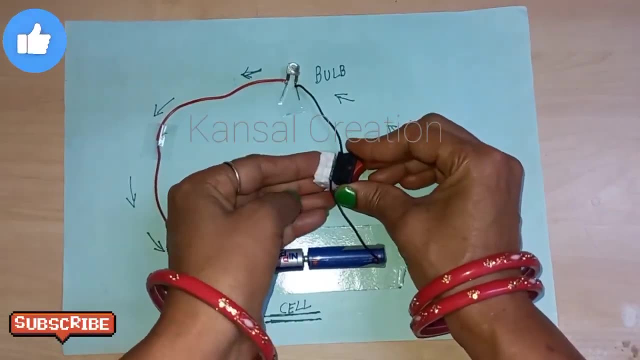 Open it up and finally explore Everything that you thought you could never do before. And even when you feel low, you can still go. Even when you feel slow, you can still go. Even when there's no hope, you can still go. I'll never answer to no man, I'll still go. 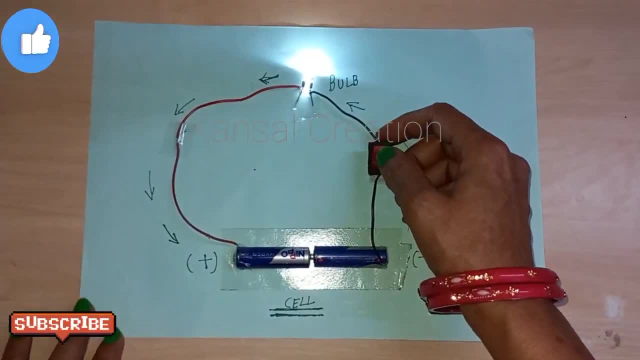 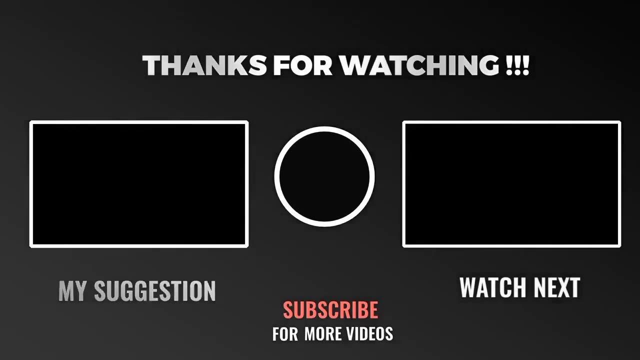 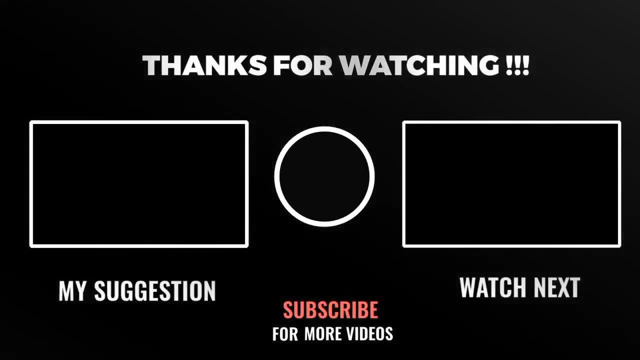